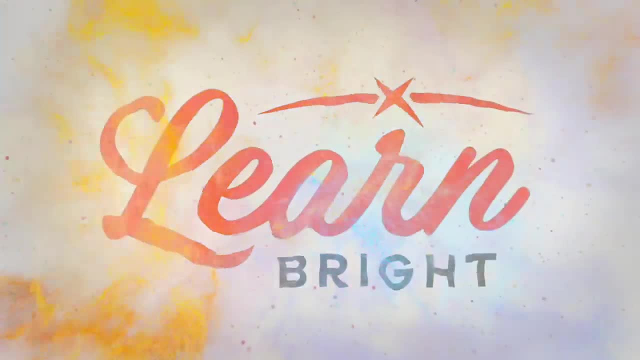 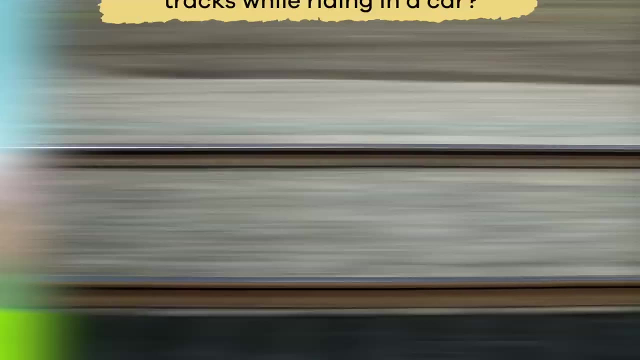 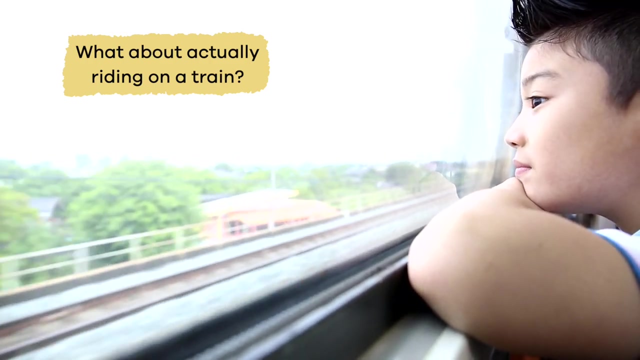 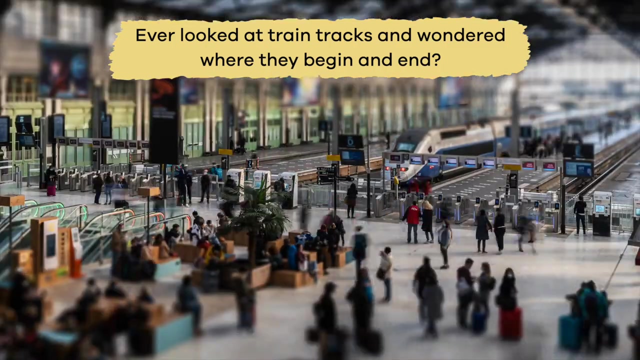 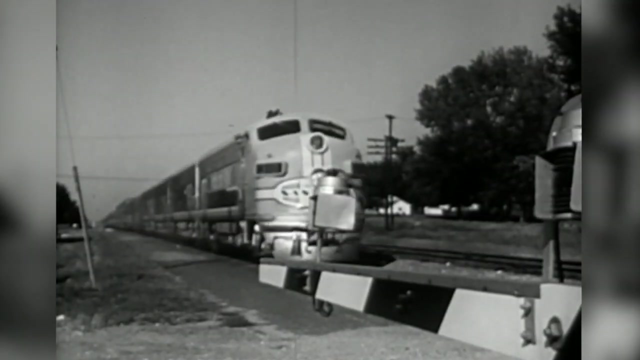 The History of Railroads for Kids. Have you ever driven over railroad tracks while riding in a car? What about actually riding on a train? Ever looked at train tracks and wonder where they begin and where they end? Well, you are in luck. Today we are going to talk all about the history of trains and railroads. 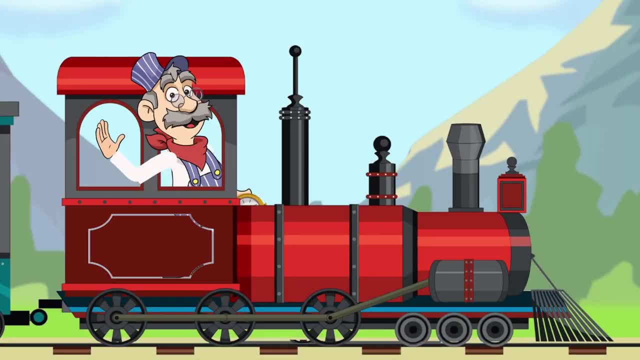 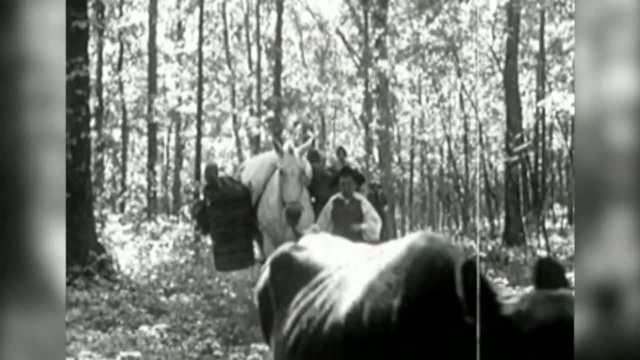 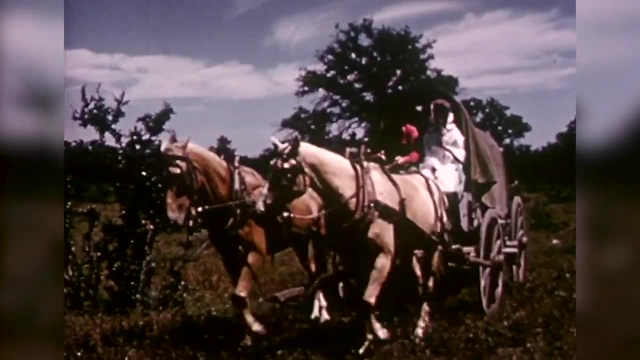 Let's meet up with our conductor and try not to lose our train of thought while we learn. Before the railroads, people traveled mainly by foot, horse or horse-drawn wagon. You know, like the pioneers. As you can imagine, this was not a very fast way to travel. 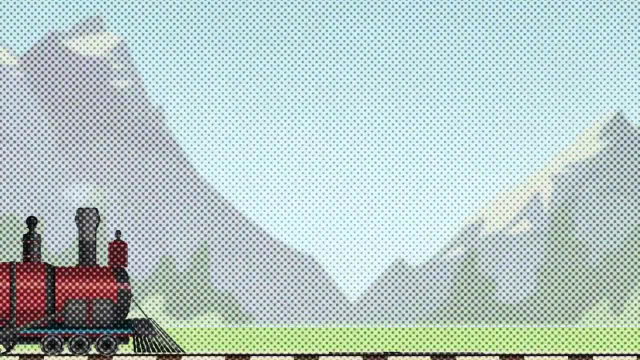 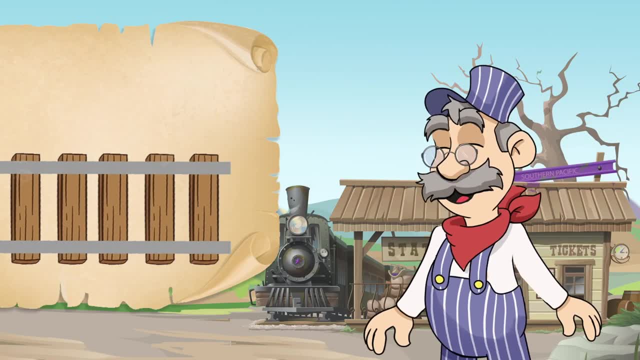 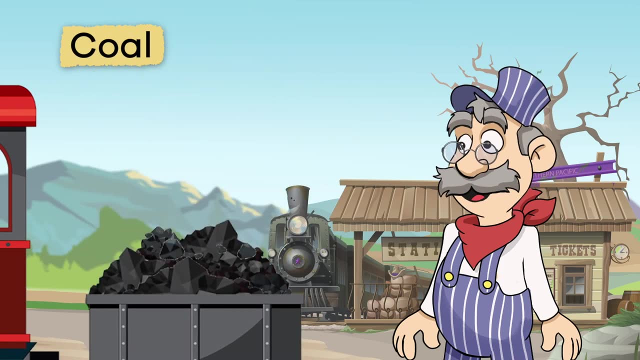 And you cannot, And you cannot take a lot of stuff with you. The first railroads were designed to carry freight or goods from place to place. Tracks were made with steel and wood or stone. The first train cars were designed specifically to haul coal, which was a main source of heat at the time. 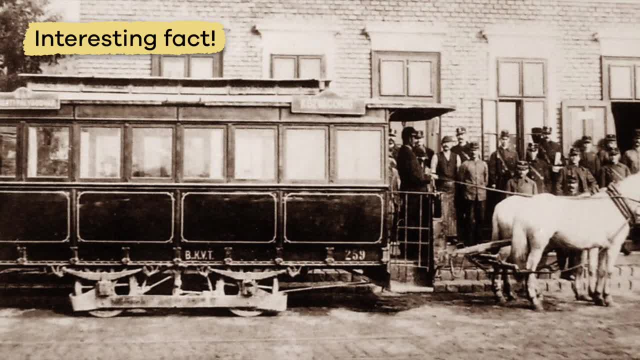 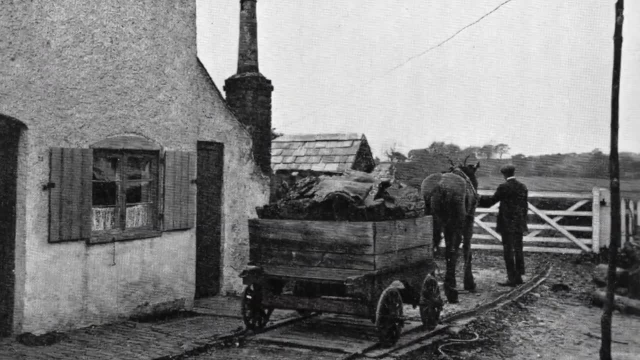 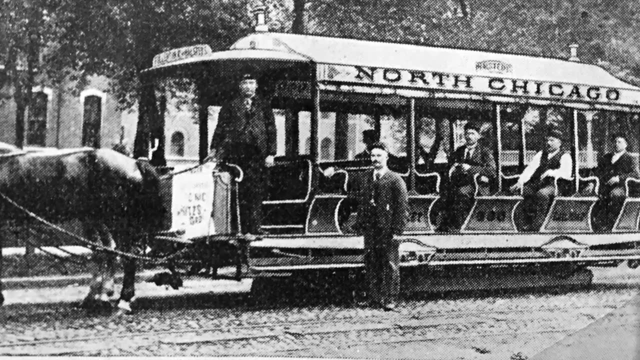 Here is an interesting fact: The first train cars were actually pulled by horses- Horses. You might be asking yourself why pulling rail cars was any faster than if a horse pulled something on a road. Well, for one thing, train tracks made the path a whole lot smoother. 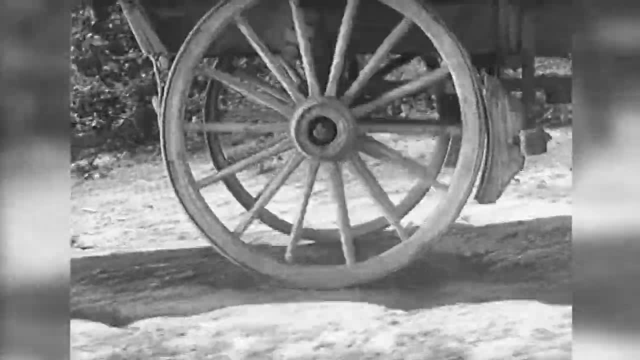 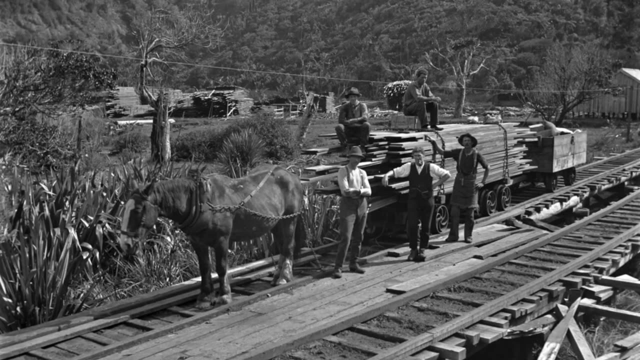 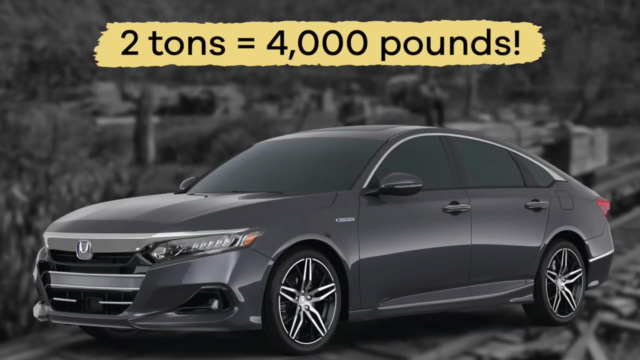 Roads were not smooth and paved like they are today. In fact, on a road, a horse could only pull about 350 pounds. On a steel track, one horse could pull as much as two tons, which is equal to 1,000 pounds. 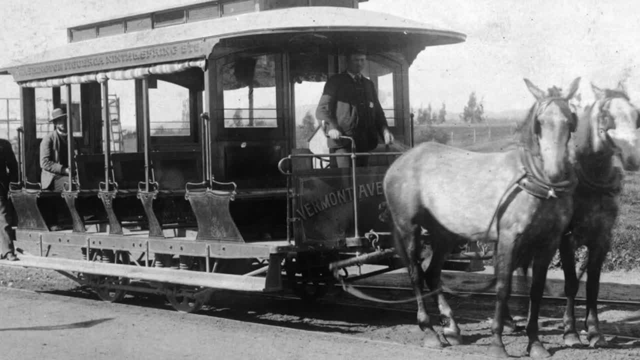 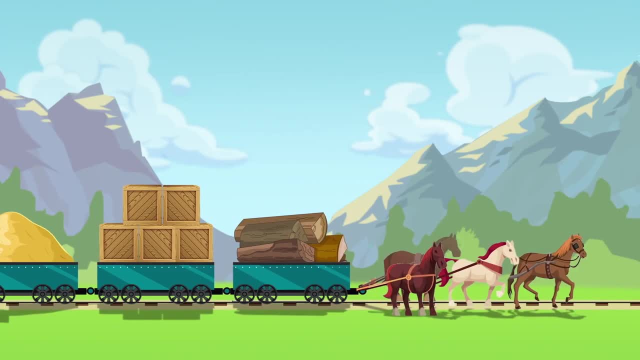 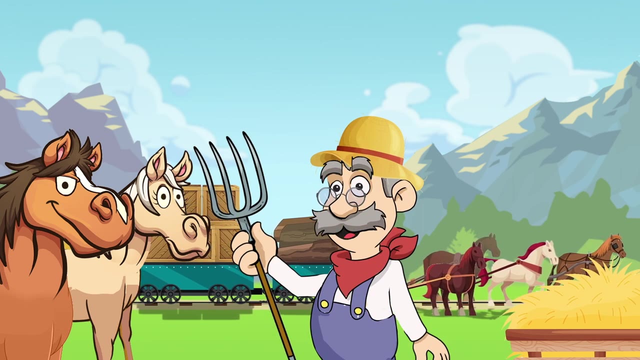 Whoa. Even though horses could carry more on a track than on a road, there were still lots of problems with using animals. For example, horse-pulled rail cars were still super slow and someone had to make sure the horses stayed healthy. 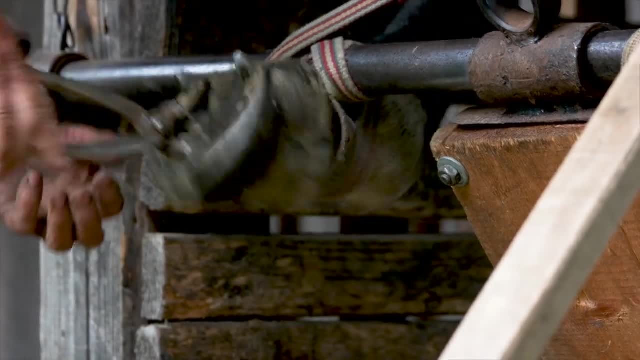 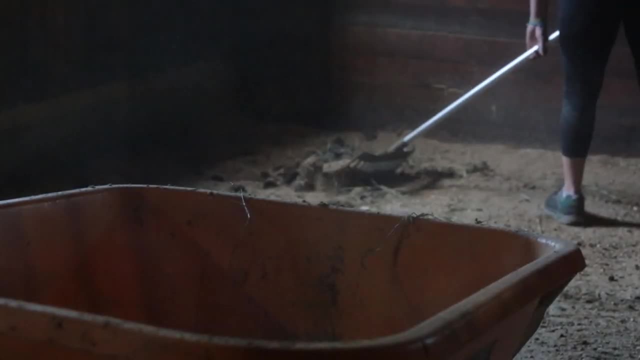 Not to mention clean up the mess that horses left on the train tracks. We would not want to volunteer for that job. We would not want to volunteer for that job. PU. The solution to these problems came in the form of steam technology. 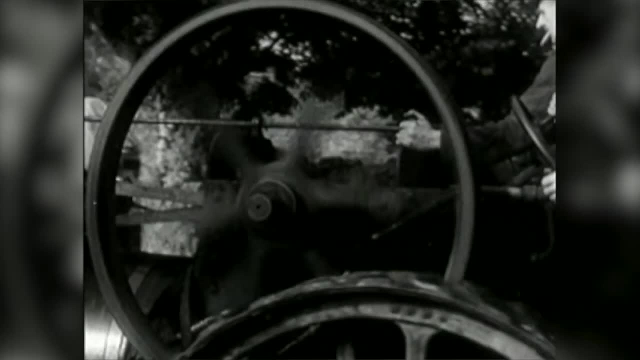 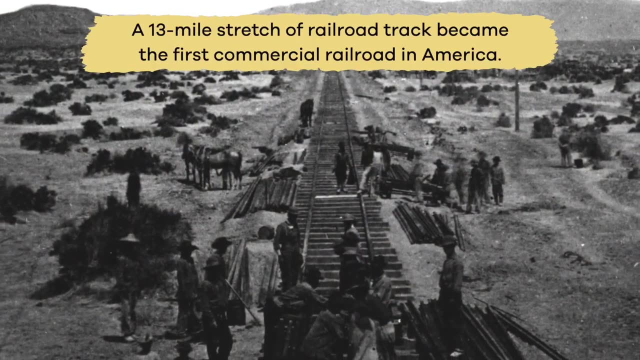 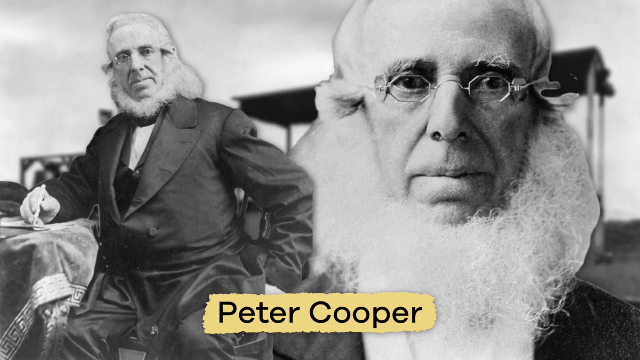 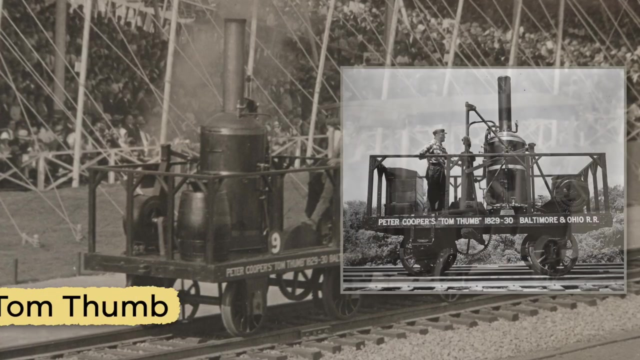 which was already being used to power other machines like steamboats. In February of 1827, a 13-mile stretch of railroad track became the first commercial railroad in America. A man named Peter Cooper successfully transported a small crew of people on a steam locomotive, affectionately named Tom Thumb due to its compact size. 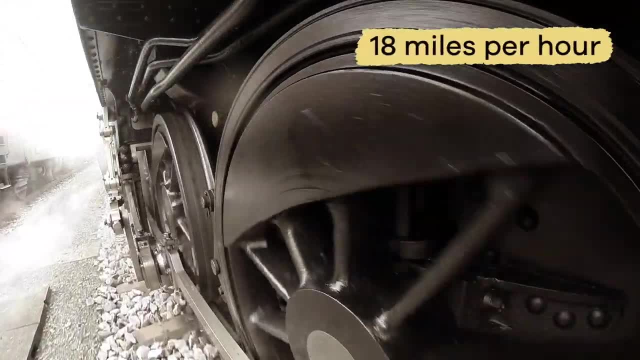 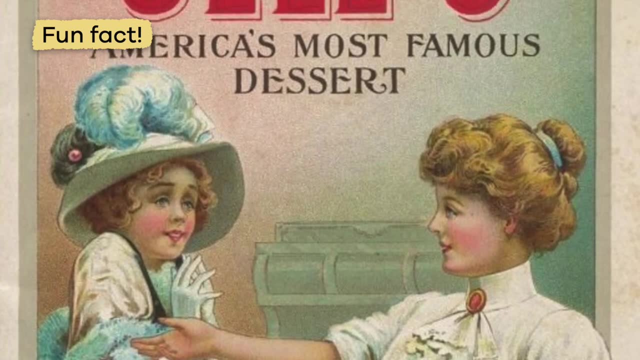 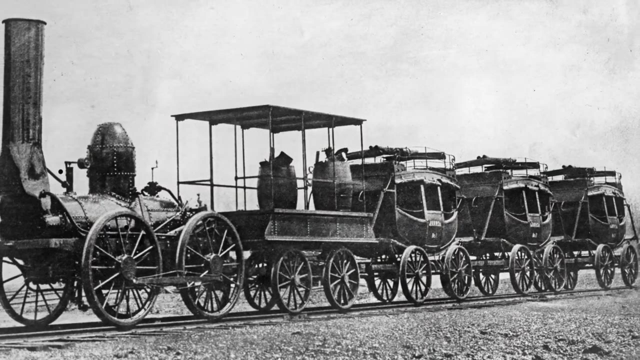 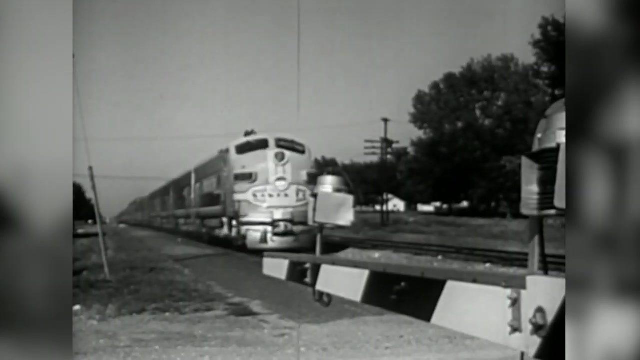 Tom Thumb went an astonishing 18 miles per hour over a curvy, hilly railway. Fun fact, Peter Cooper is actually best known for inventing Jell-O. It was not long after the Tom Thumb's ride that entrepreneurs or business people saw the potential to make lots of money on expanding railroads to every major city. 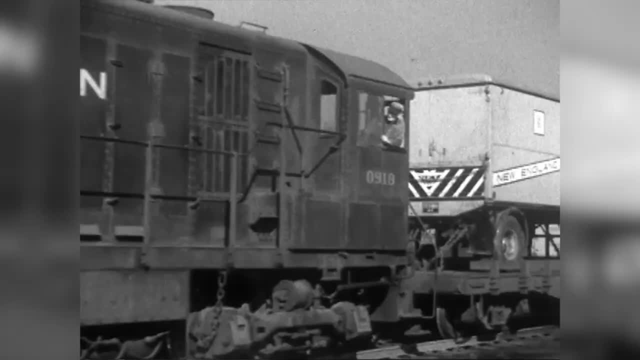 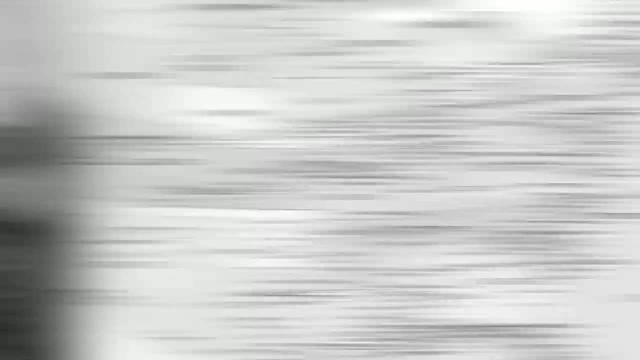 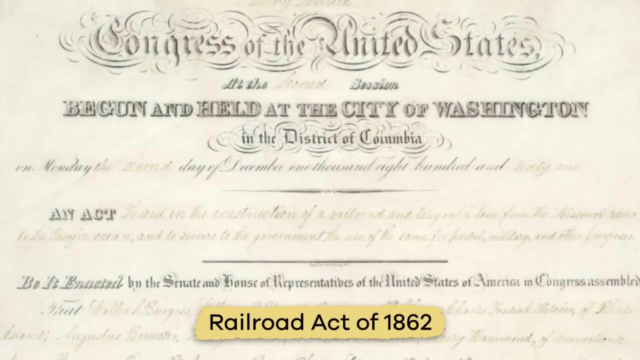 in the United States, Finding a better way to transport goods, mail and people West became a huge priority, especially a railroad that connected the Atlantic coast with the Pacific coast. The Railroad Act of 1862 paved the way for joining East and West by railroad. 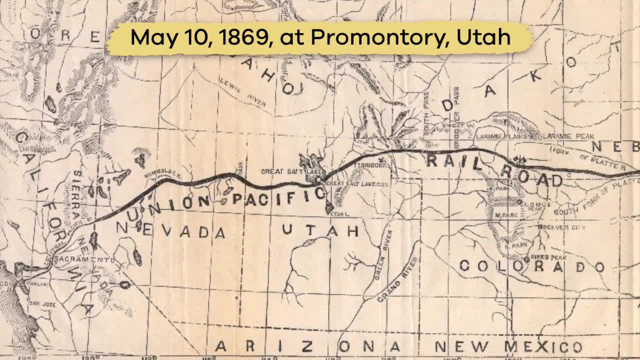 and the first railroad to be built in the United States. The railroad act of 1862 paved the way for joining East and West by railroad and, on May 10, 1869, at Promontory Utah, the two railroad companies Union Pacific Railroad. 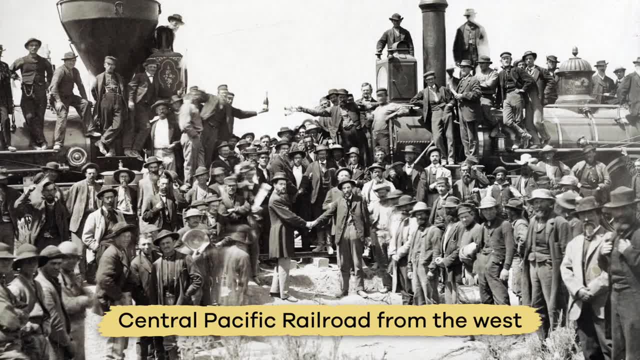 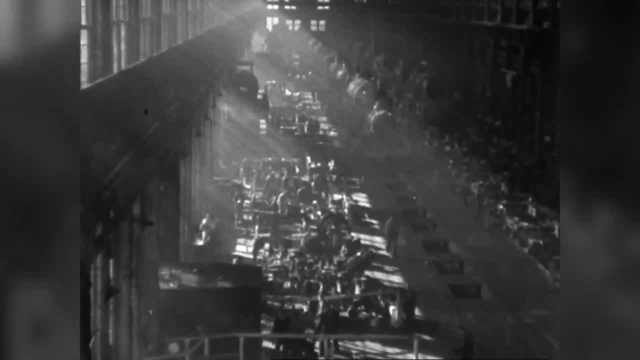 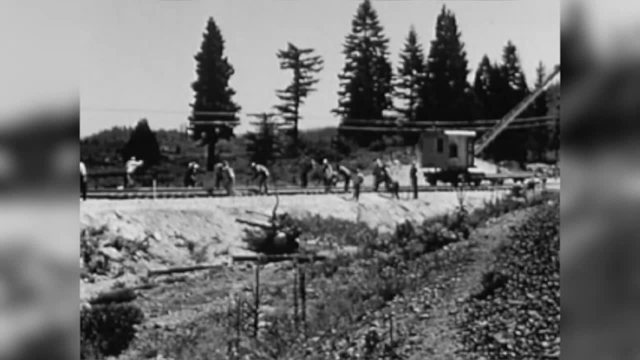 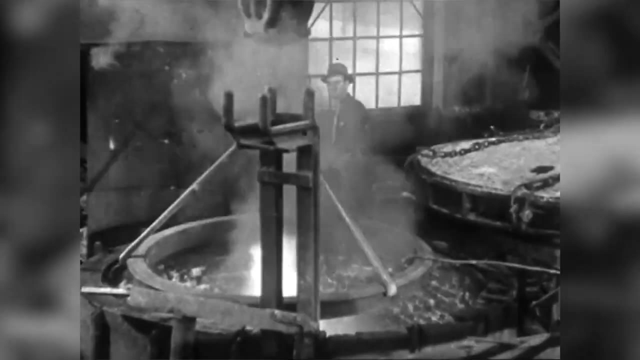 from the East and the Central Pacific Railroad from the West hammered the final spikes into the East-West rail lines. All of this railroad building was great economically for many industries. For example, thousands of construction workers were needed to clear land and lay rail tracks. Steel companies also employed thousands to make the steel for the rails and parts for the. 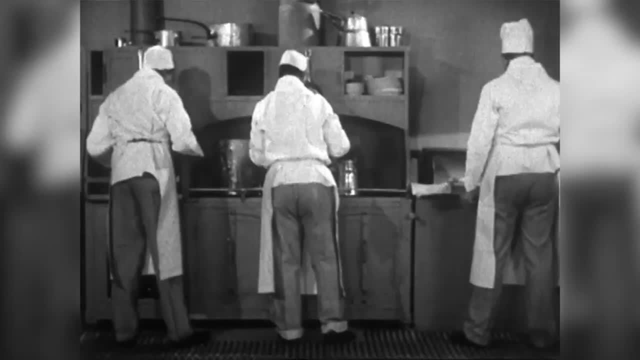 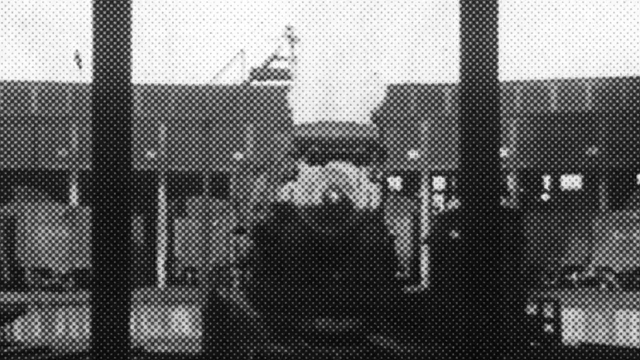 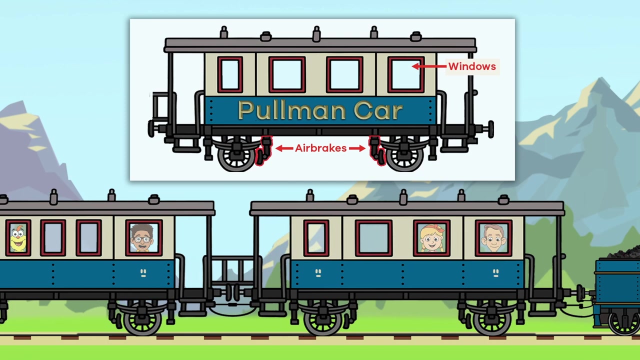 trains. Lumber was also needed and supplies to feed the workers, And so towns sprung up. everywhere, a railway was being built. Innovations like the air brake, the Pullman car, which was the first passenger car to have windows, and the addition of springs all helped make rail travel.